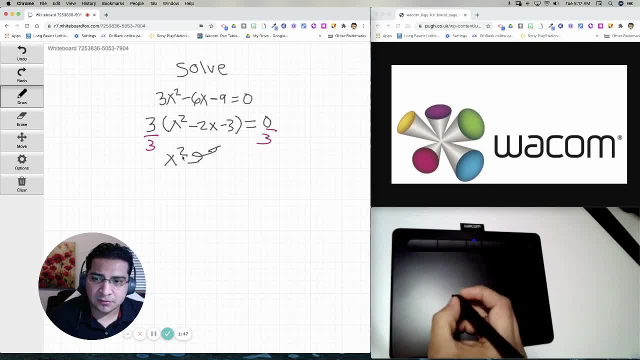 So I'm only left with x squared minus. oops, Let me just undo that. Hey, pretty easy. Hey, that was a good mistake to make. Minus 2x minus 3 equals to zero, All right, and then I can just factor this right here: 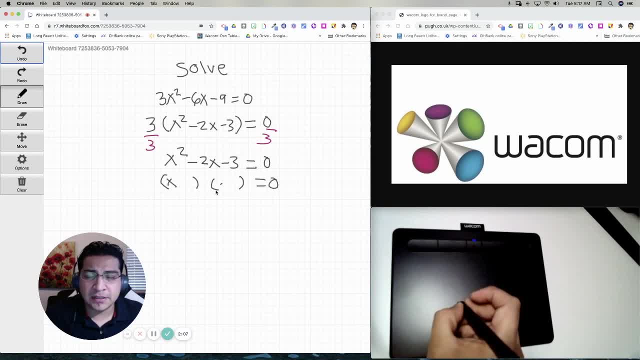 Okay, so I can do x times x factors of three. that will give you a negative 2.. So that's going to be 3 and 1. And I'm going to put negative here and positive here. That looks like it's going to work. 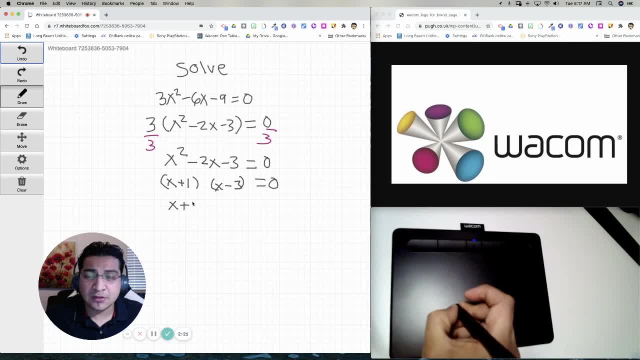 Now I can set each of the factors equals to zero. So x plus 1 equals zero, And x minus 3 equals to zero. So this will be minus 1 minus 1.. And so I'm showing every single step so that you guys can see the beauty. 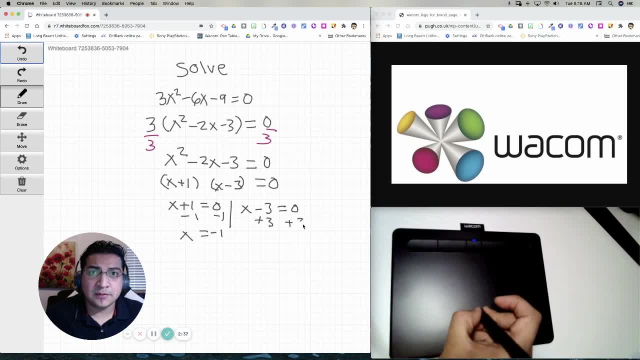 of using the tools here. So plus 3 plus 3 x equals to 3,. okay, And that is how you do this problem. Now, those are the zeros. okay, Those are the zeros. If I want to do a quick sketch of this, I can actually do it. 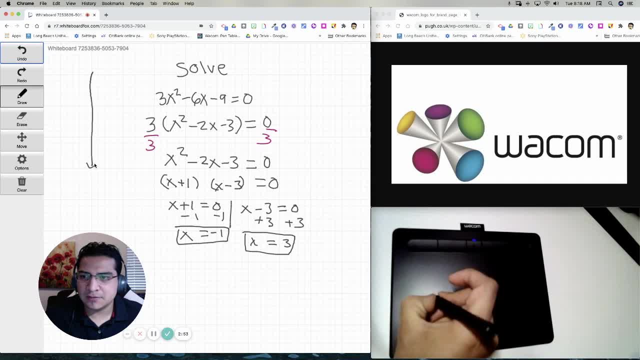 over here. This shouldn't be that bad, you guys. This parabola opens up right And it looks like the zeros are negative, 1 and 3,, so 1 right here. Just put 1 right here, And the other one is 3, so 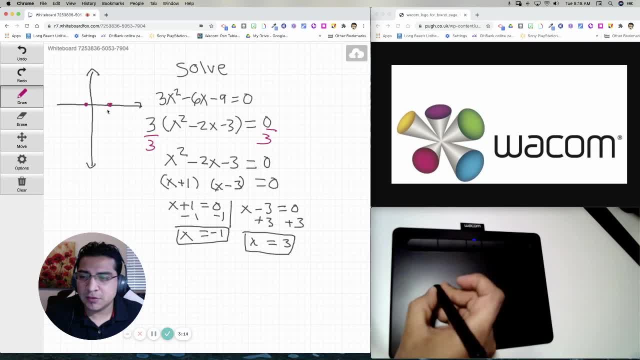 1, 2, 3, right there. They do have an axis of symmetry right in the middle there, so that's going to be 1, 2, 1, 2, so like: right here, So I can draw my axis of symmetry. 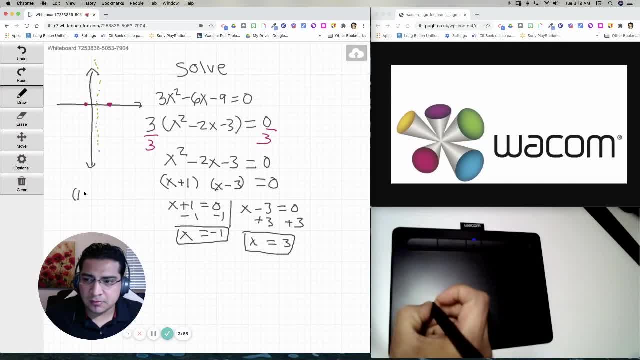 Alright, and then I'm going to plug in 1 square minus 2 times 1 minus 3.. And let's see what we get. Okay, so this will be y equals and that's going to be 1 minus 2. 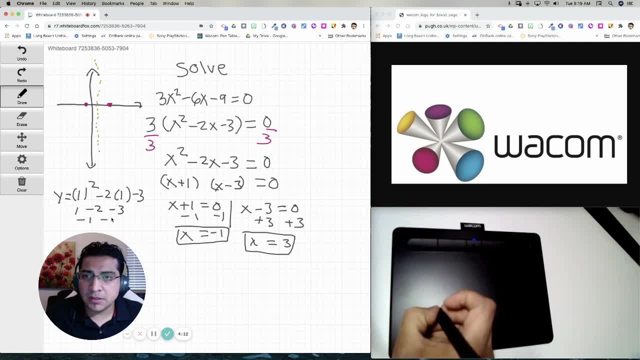 minus 3, and that's going to be minus 1 minus 3, and that will give us negative 4.. So the minimum point of this parabola is going to be negative 4, so let's go ahead and go down 1.